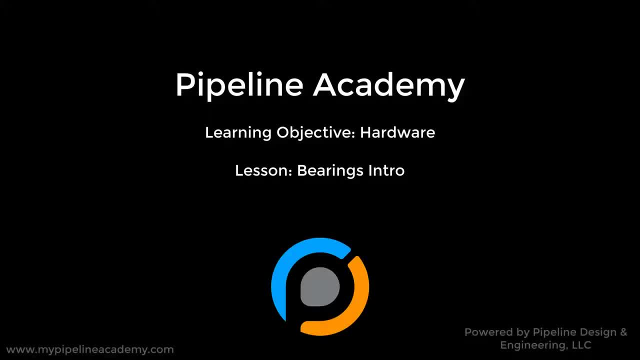 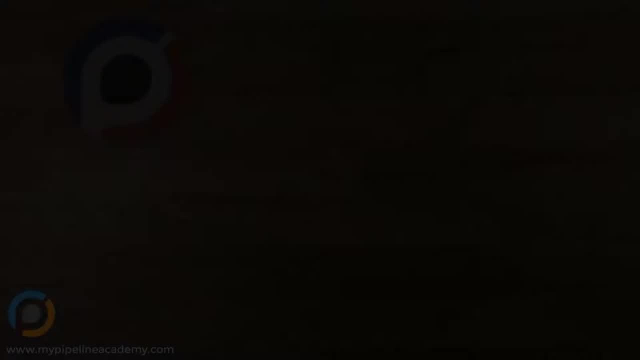 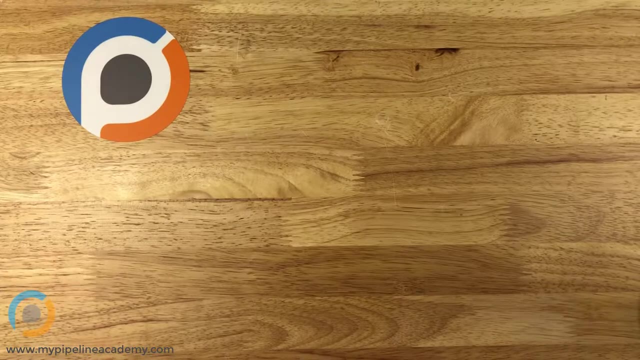 What kind of hardware would you use if you had to facilitate very, very smooth rotation and maybe even high speed rotation, high RPM? What hardware could you use to facilitate that rotational motion? You don't want any slop or play or wiggle in that motion. You want it to be. 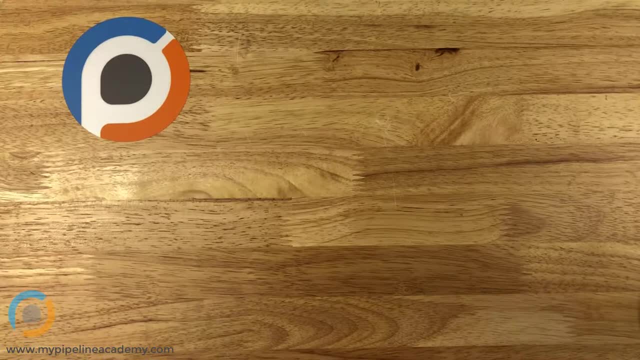 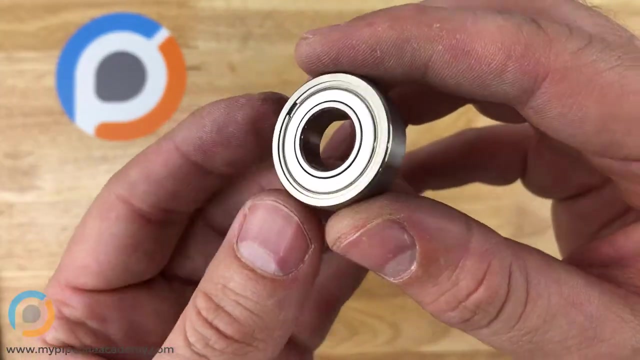 very precise. What could you use? Well, the answer is ball bearings, And there are a few different kinds of ball bearings that we're going to look at Here. this one is maybe the most common type of ball bearing. It's just a round ball bearing. There are balls inside of this and you can't see. 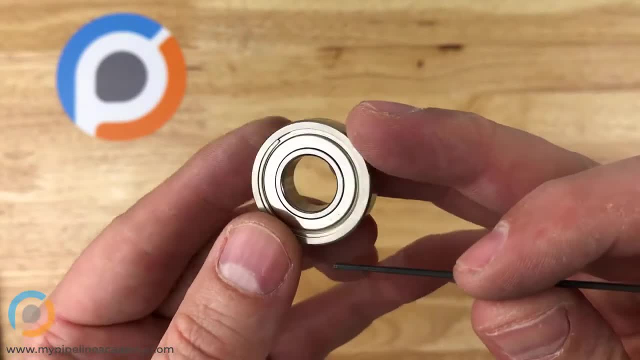 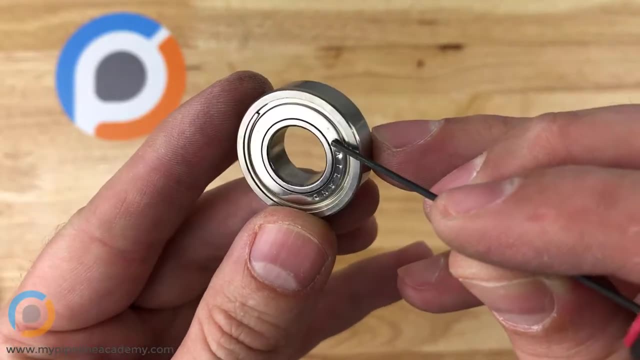 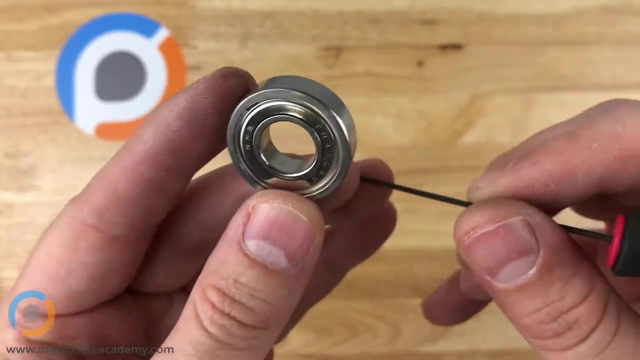 them because they're shielded. This is a shielded style ball bearing, But in here, all the way around, there are little balls that allow this to spin really smoothly and with very high precision. This is some anatomy of a ball bearing. This is called the outer race. 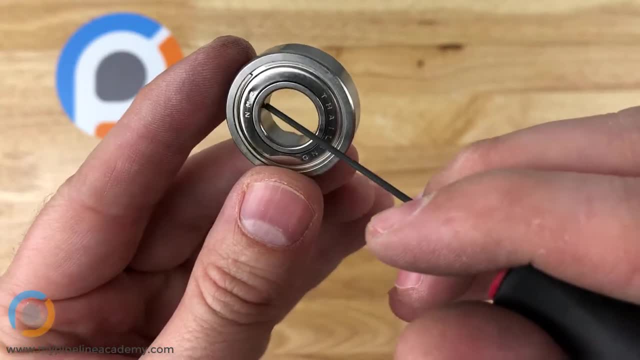 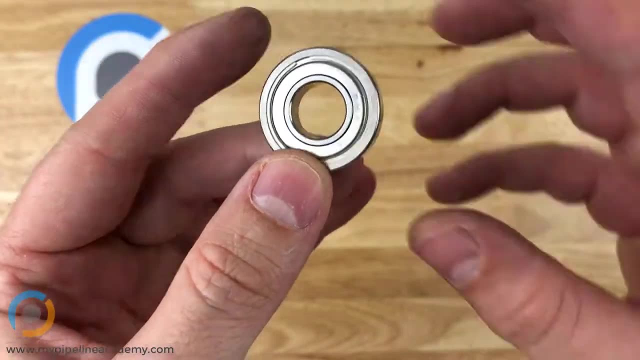 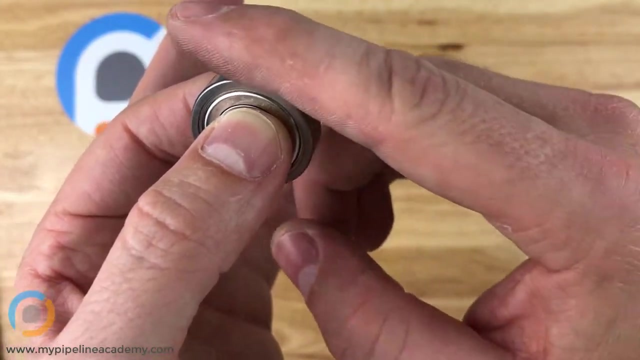 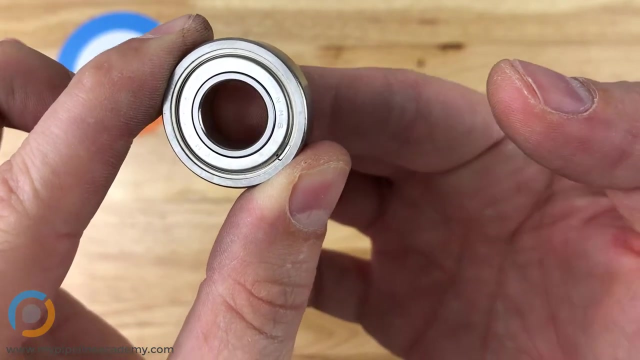 R-A-C And this is the inner race, And the two- the inner race and the outer race- rotate relative to each other. So if I kind of hold that inner race and prevent it from moving, I can spin the outer race. Likewise, if I hold the outer race, I can spin the inner race. And it's a very, very 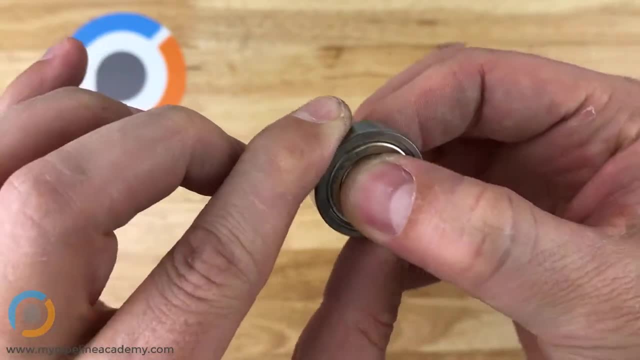 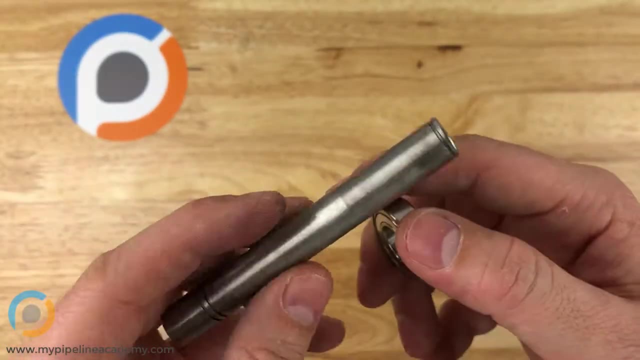 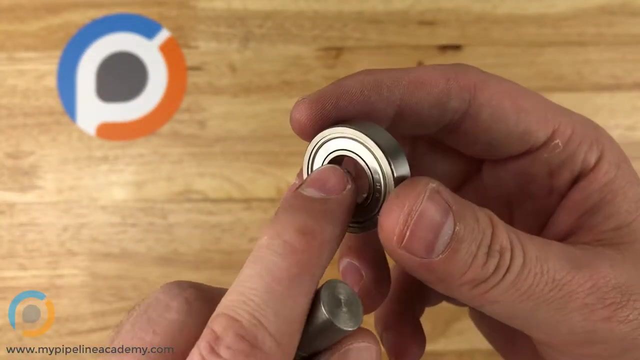 smooth, very precise rotational motion. There's no wobble Or play in there, And you typically use a bearing on a very high precision shaft or axle or rod. So this particular ball bearing has a one-half inch diameter inner race, And so it's meant to be used with a shaft that has 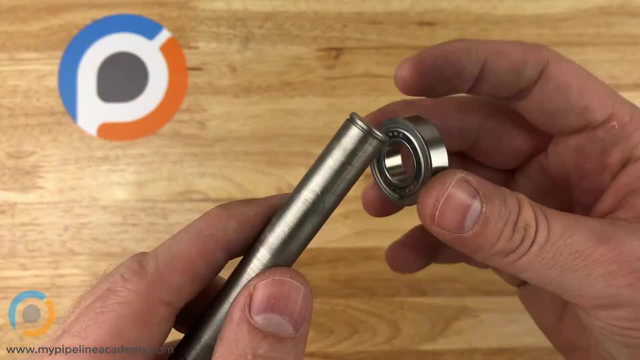 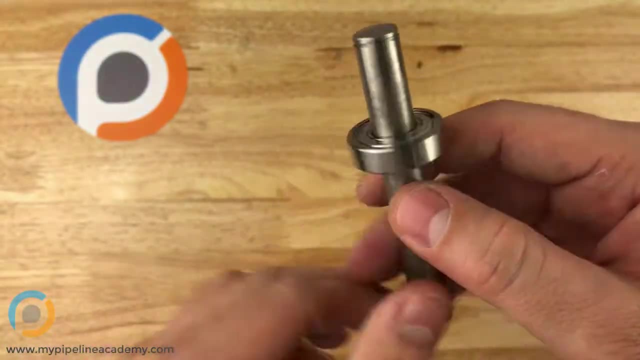 a half inch diameter And this shaft does have a half inch diameter So you can slide this on. It's a very nice, smooth fit. In fact, I would say that this shaft is maybe even a little bit undersized. I would, I would want it to be a little bit tighter. I can feel just a 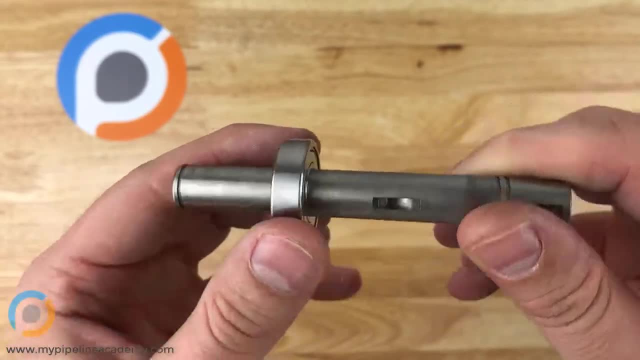 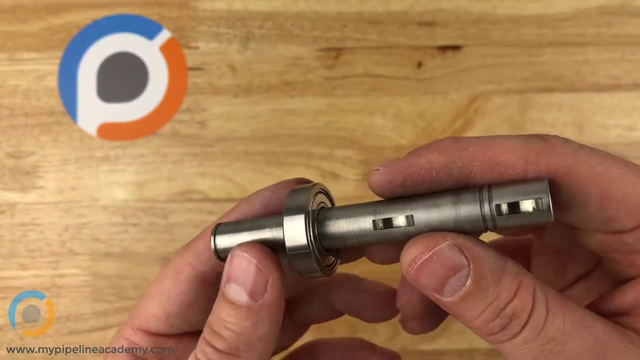 small hair of play a wiggle in there. so ideally, this shaft is going to be a little bit bigger, and when I say a little bit bigger, you know we might be talking less than 1,000th of an inch bigger, maybe five, ten thousandths of an. 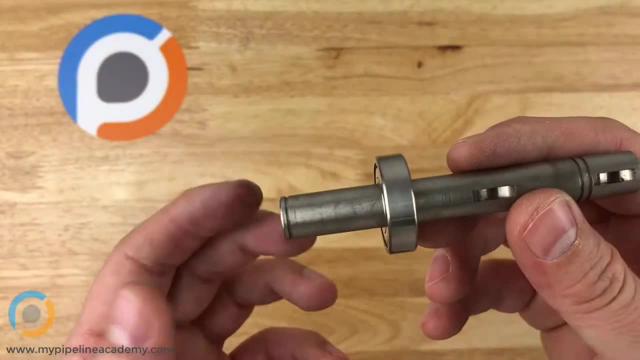 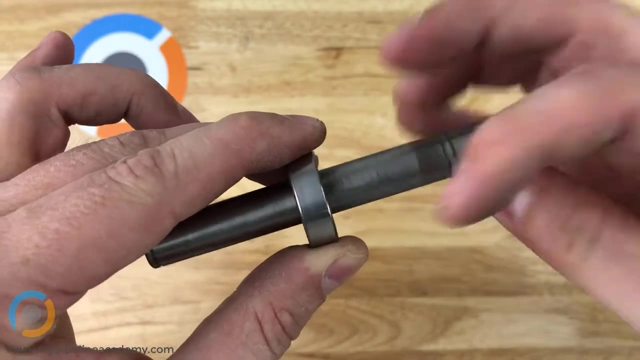 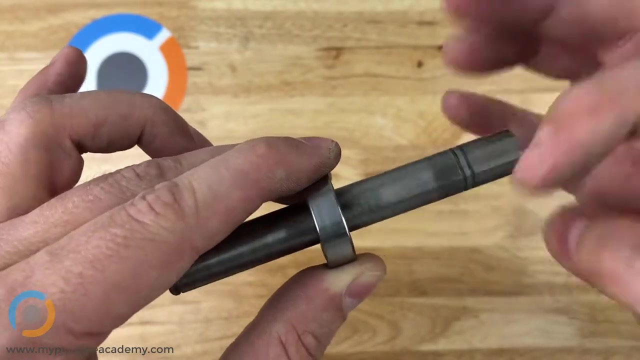 inch bigger, or seven or eight, ten thousandths of an inch bigger, something like that. anyway, it's pretty close and you can see that you know this facilitates this really nice smooth motion. you use bearings a lot with I don't know axles that are, you know, turning in gears or something like that. 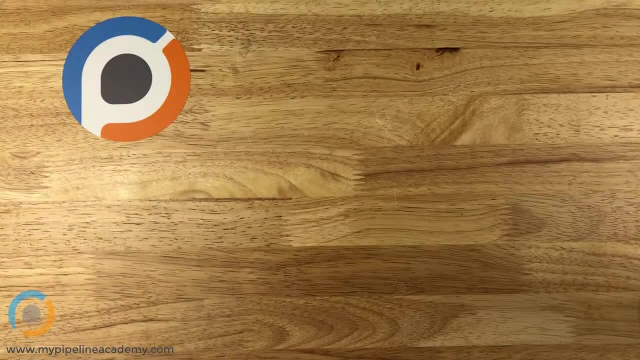 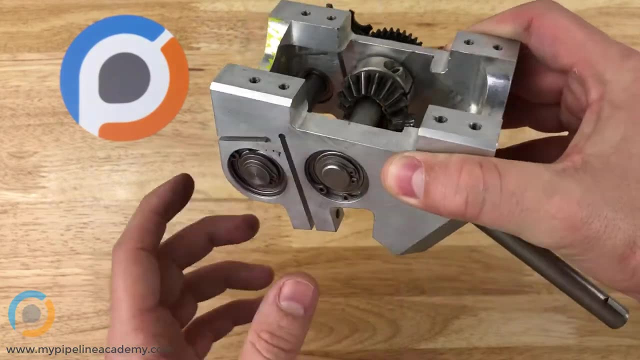 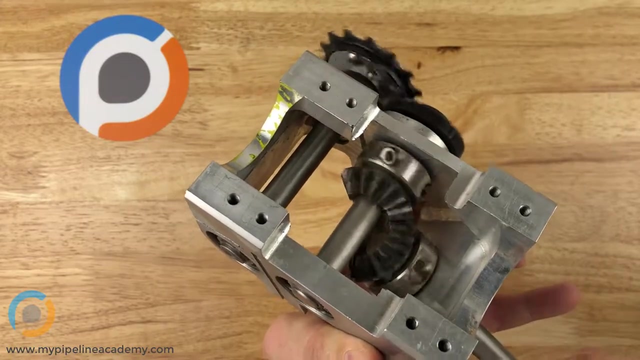 in fact, we're gonna look at this in a CAD video, but this is an actual little gearbox that we designed. you can see we've got a few different types of gears in there. we won't go over the exact gears, but they're all this. this motion is very 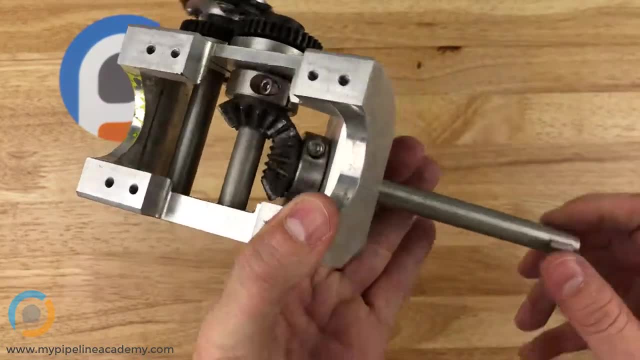 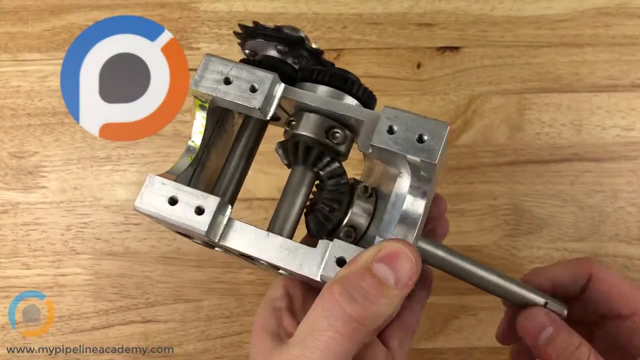 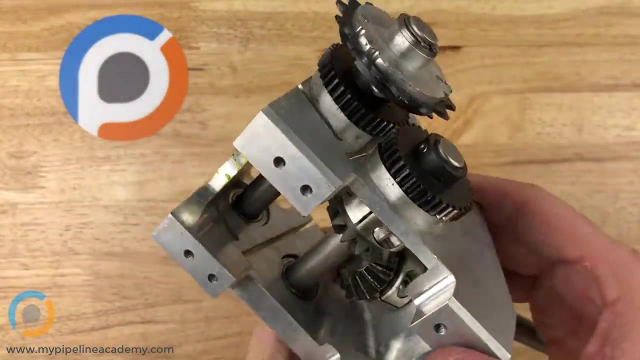 smooth every. there's very little resistance. I'm spinning this shaft and it doesn't require hardly any force, hardly any torque, just spins really smoothly and everything's very smooth, very, very well controlled and the the reason we use ball bearings in here is because we have two gears that need to. 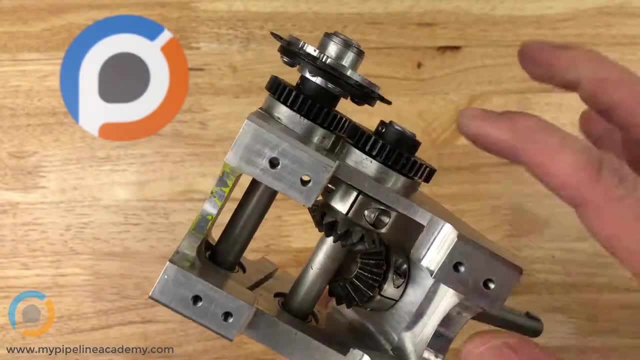 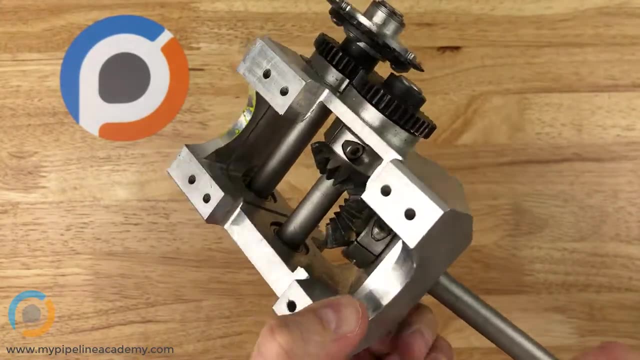 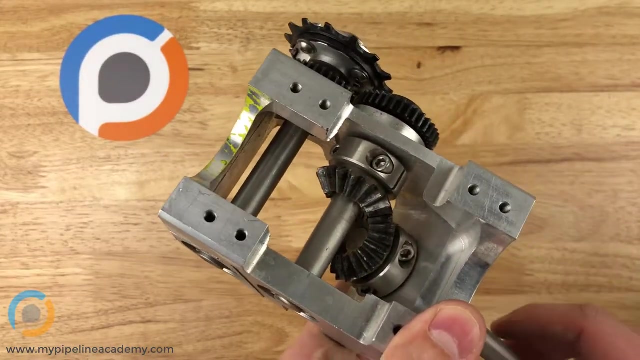 to mesh their teeth need to mesh together actually two sets of gears that need to mesh their teeth need to mesh together actually two sets of gears- spur gears- over here, and over here we've got some some bevel gears or miter gears, and gears require very, very accurate relative placement, relative you. 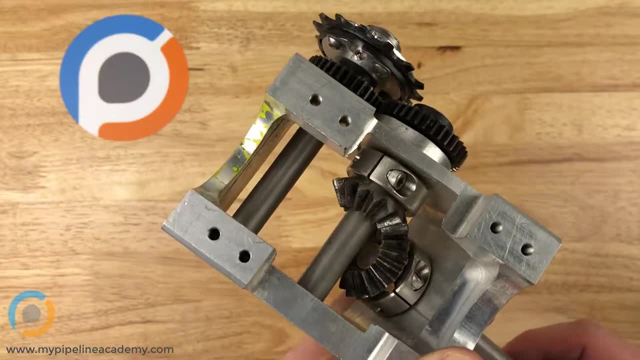 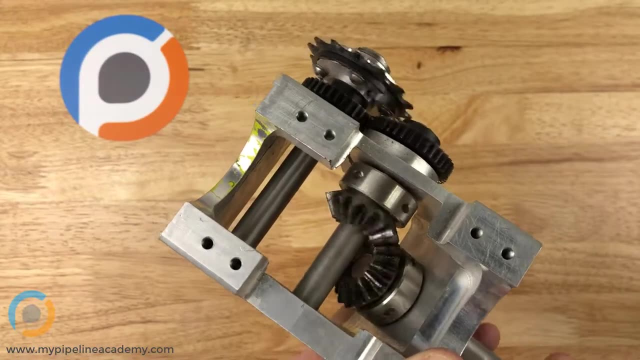 know one geared to the other, and if they're they're not placed extremely precisely, then the the gears will wear faster. they'll they'll make more noise and they'll they'll transmit less noise and they'll they'll transmit less noise and they'll they'll transmit less torque. so it's important the gears are. 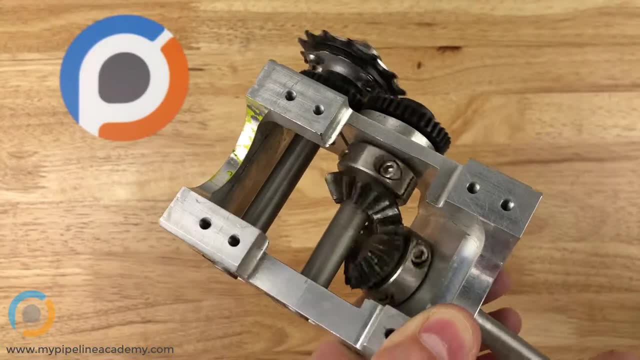 less torque, so it's important the gears are less torque, so it's important the gears are placed very, very precisely relative, placed very, very precisely relative, placed very, very precisely relative to one another. and the way that you do that to one another and the way that you do that 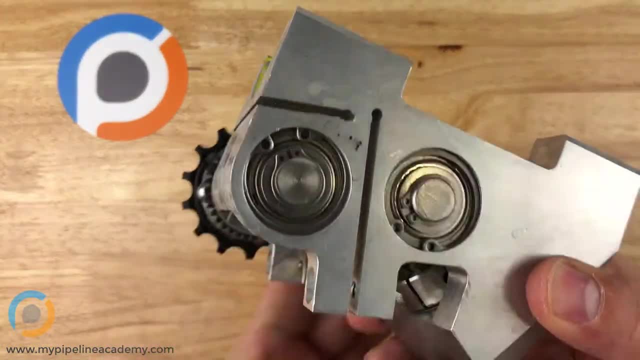 to one another, and the way that you do that is in part by using ball bearings. so is in part by using ball bearings. so is in part by using ball bearings. so you can see, here we've got a ball bearing. you can see, here we've got a ball bearing. 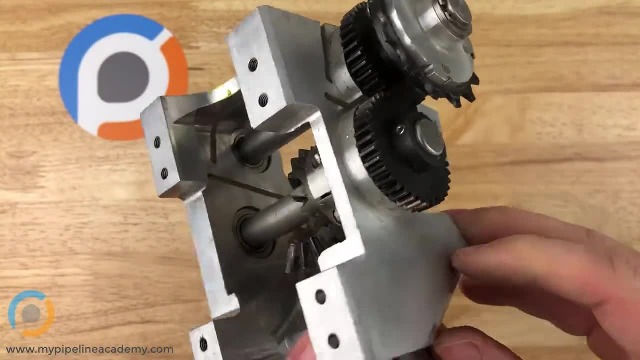 you can see, here we've got a ball bearing there and there, and then on the there and there, and then on the there and there, and then on the other side it's a little bit harder to see, other side it's a little bit harder to see. 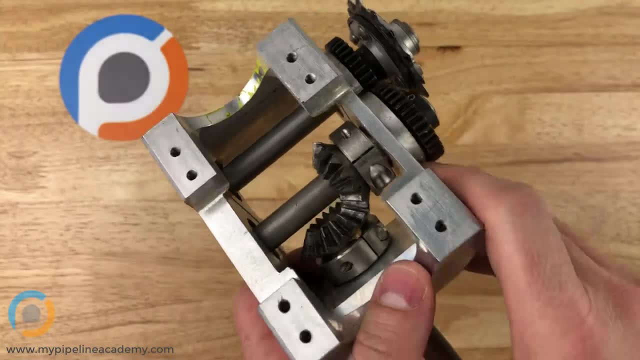 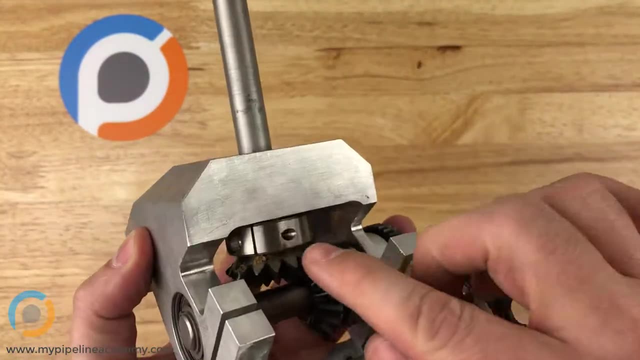 other side it's a little bit harder to see, but there's another ball bearing in here and one in here, and then we have our our input shaft right here. we've got one ball bearing there and there's a second one that you can't see that's in here and that allows our input shaft. 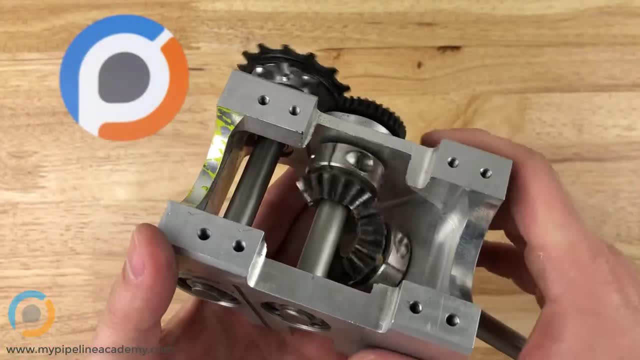 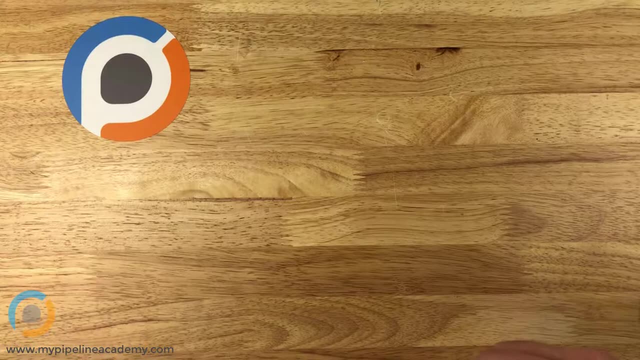 to move really smoothly. so there's an example of of how some gears are used. now there are a few other kind, i'm sorry. an example of how ball bearings are used. i'll show you a few other examples here. this guy is a pulley actually you can see like that little v groove on there, but you 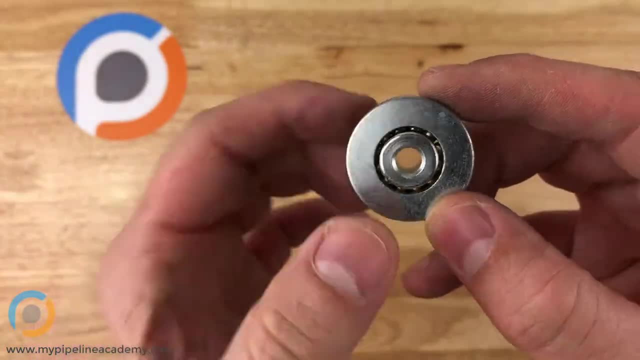 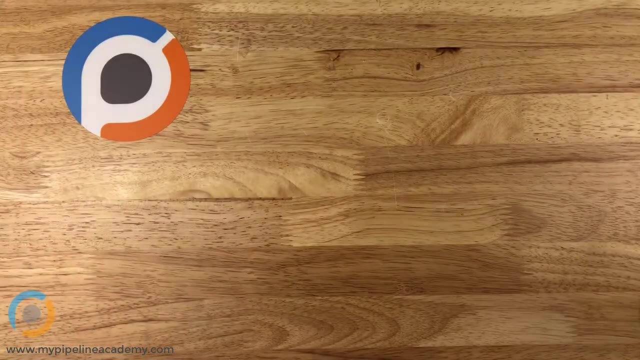 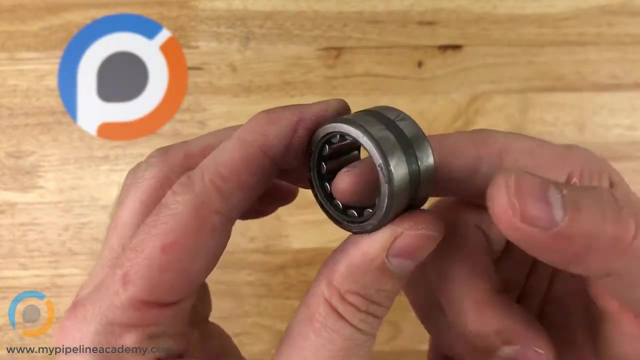 can see the ball bearings inside. you can see them reflecting in the light and you know this one spins just like any- any ball bearing, so there's some bearings in there. this is a needle roller bearing, so instead of balls there are they're basically pins inside there that that spin within. 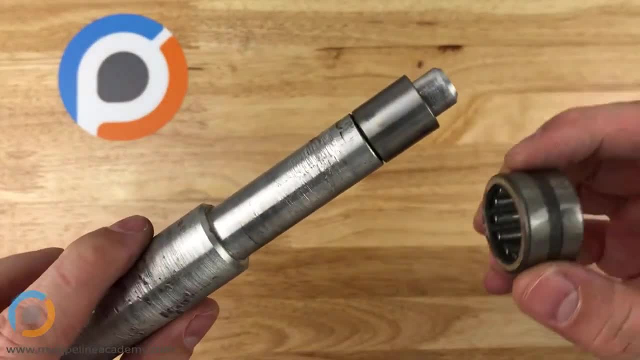 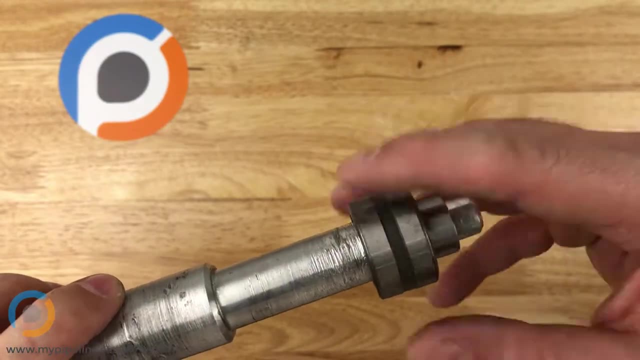 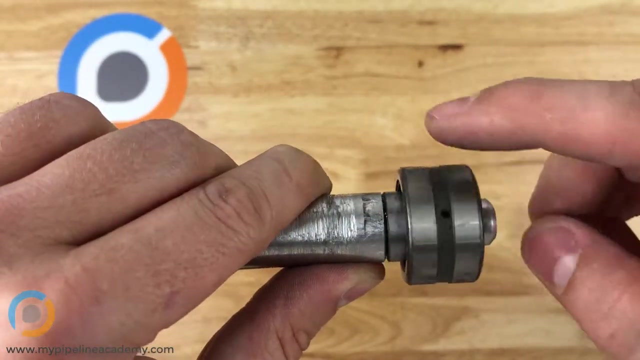 a cage and- and here is a part that that we might use with this needle roller bearing- just spins on there. now, of course we wouldn't want it to be shifting axially back and forth like that we'd we'd do something to prevent axial movement and, just you know, facilitate some nice rotational. 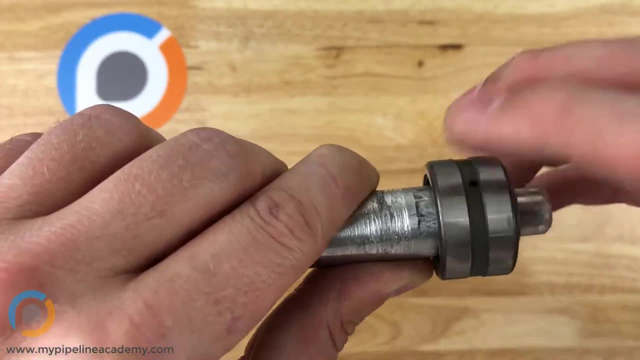 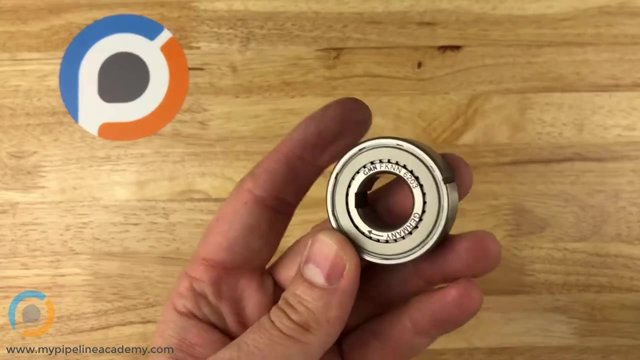 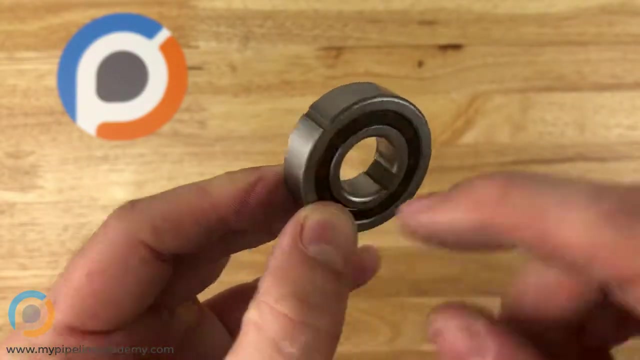 movement like that. this needle roller bearing is a little bit old and it doesn't spin quite as well. and here is another example. this is a one-way bearing and you can see that there's a little a keyway right there, a notch and another notch over there. oftentimes these, these bearings are used with, uh, with little keys. one half of the. 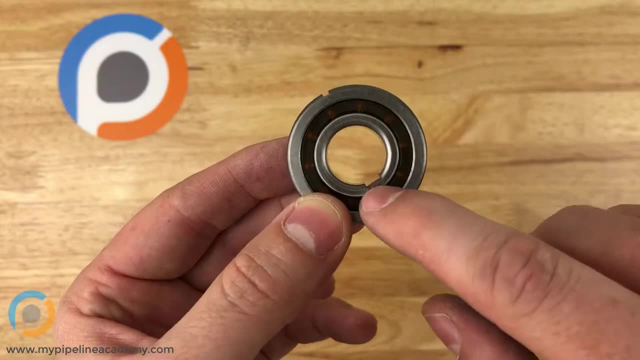 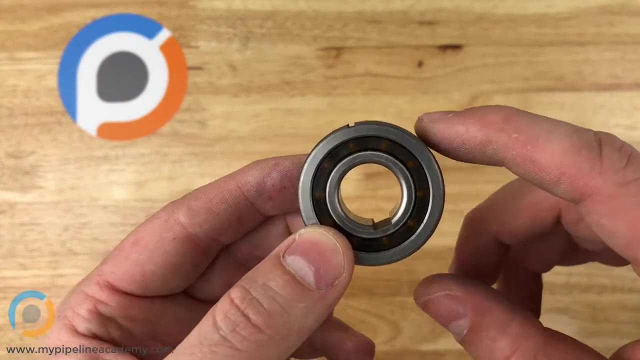 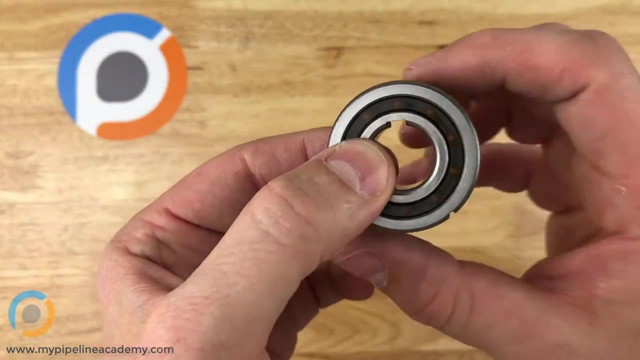 key goes into your shaft and the other half of that key goes into the notch in the bearing in the inner or outer, inner or outer race and and that locks the inner and outer race relative to whatever it's installed in. and so you can see- let's see if i get that key up here. 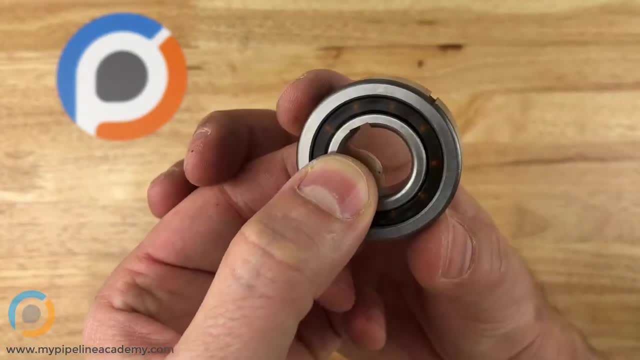 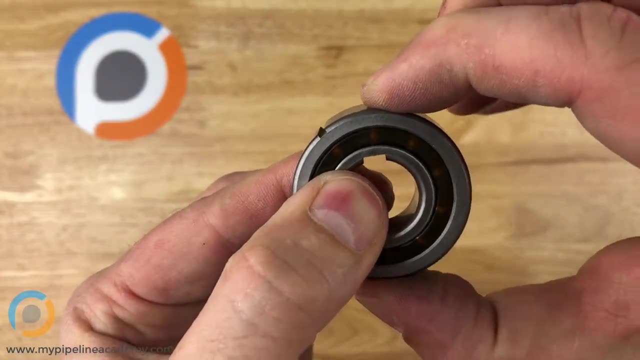 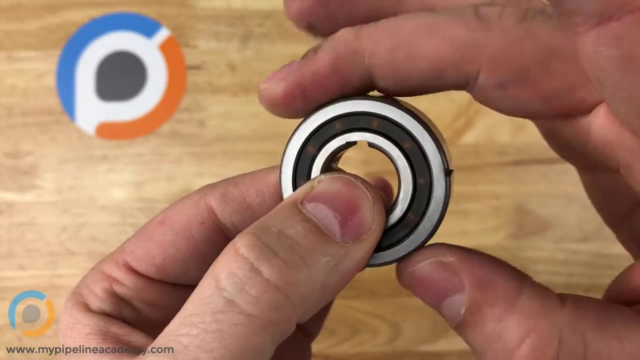 and the other keyways. on the outside you can see that it rotates. you know, no problem in that direction, right, but if i try to go the other direction, it won't move. it locks, and so these one-way bearings are just another type of bearing that can be used. 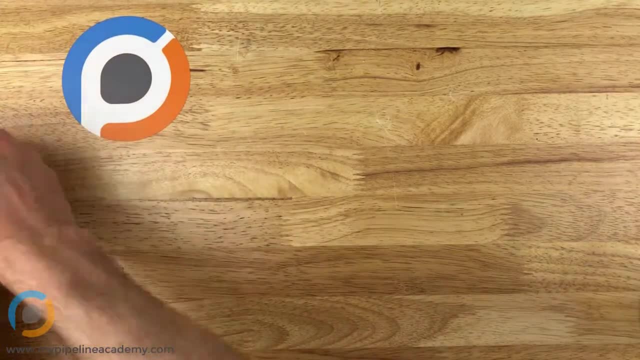 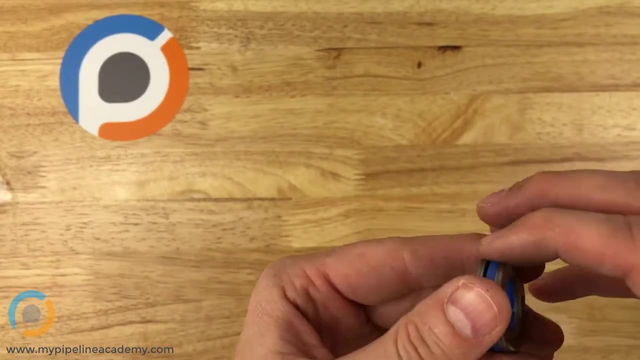 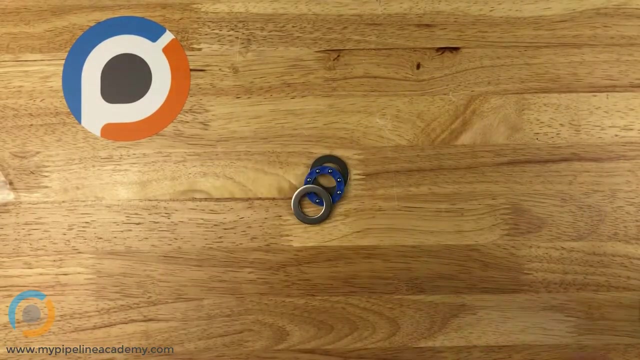 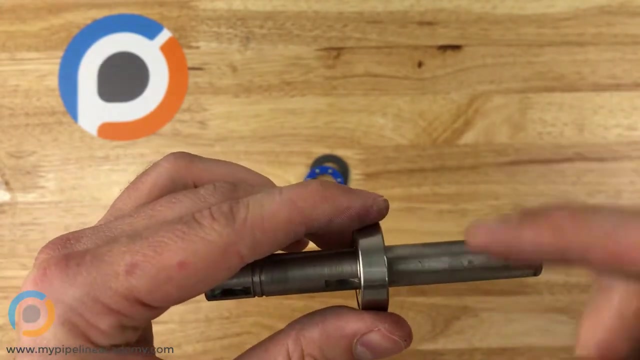 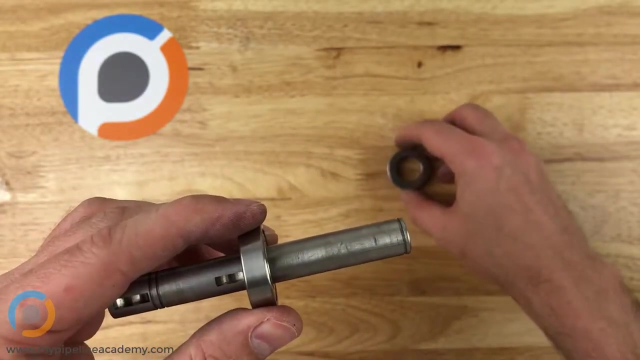 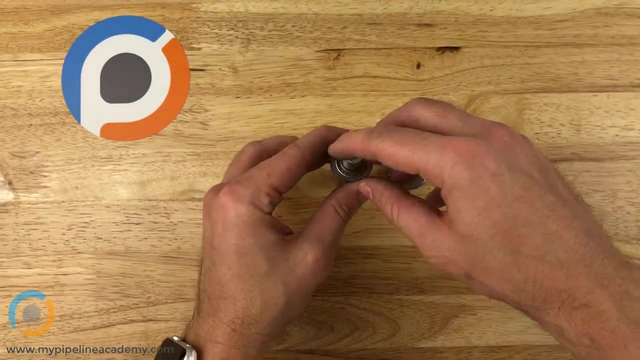 yeah and uh. last thing that we'll look at here, this is a, a thrust bearing. so the the bearings that we've looked at to date, or far. let's see transmit. how do I say this? they have the rotational motion is around this axis, whereas a thrust washer, or thrust bearing the rotational motion. let's see the rotational. 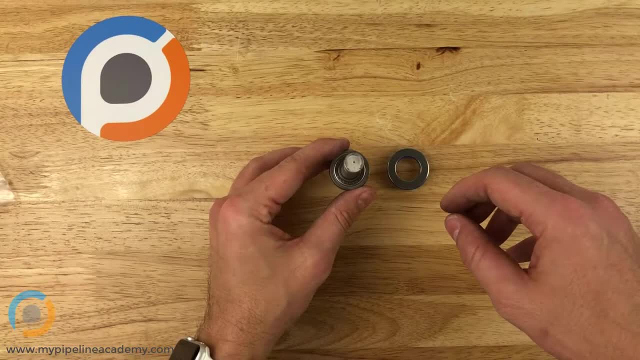 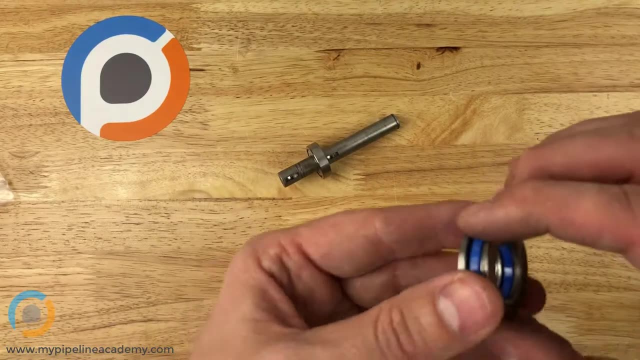 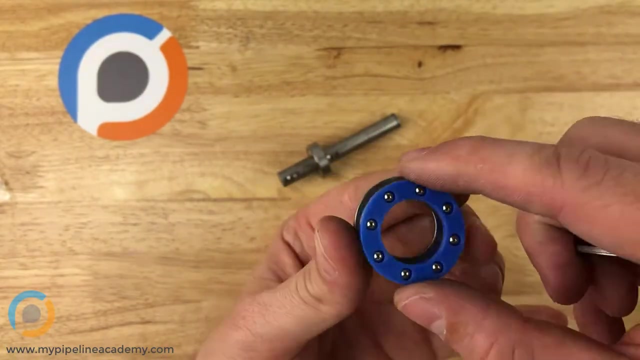 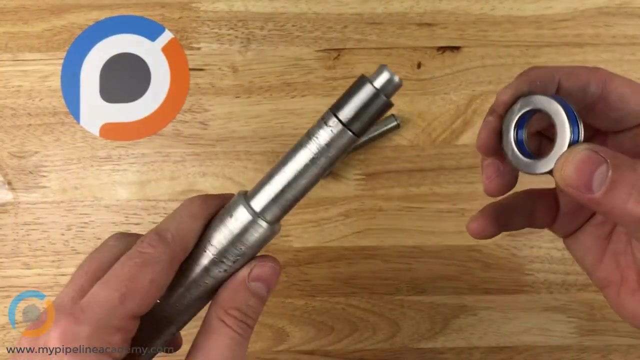 motion is the same. well, not not exactly sure. the best way to explain the difference maybe just visually. right here are the balls inside this little plastic cage. you have a metal washer on the bottom and another metal washer on top, and let's see, this is not necessarily meant to. 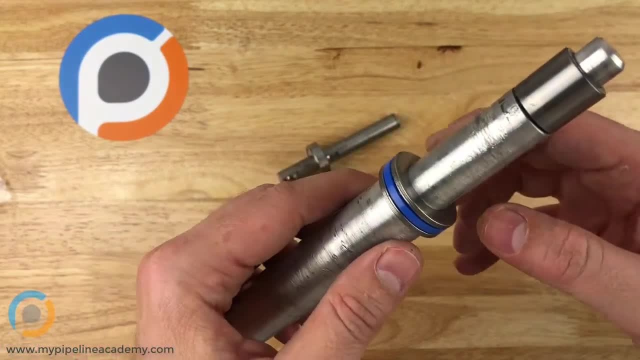 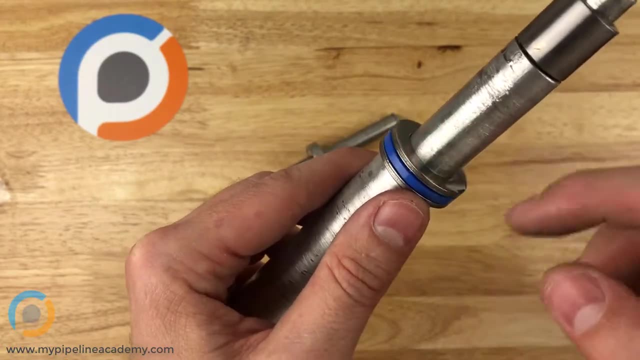 install, but just to give us something to hold it with. you know that, that's that that bottom washer is going to stay where it is and the top washer is going to move really smoothly and and you would have something on top of this top washer, something that was bearing down. 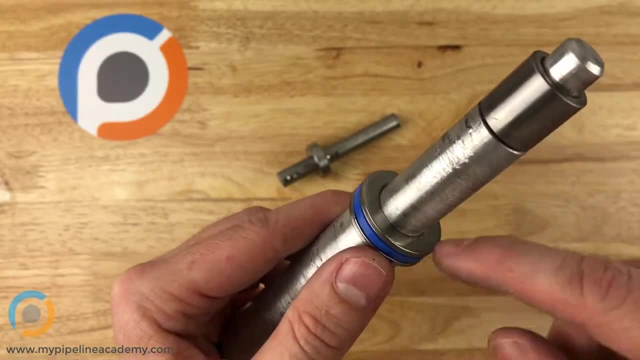 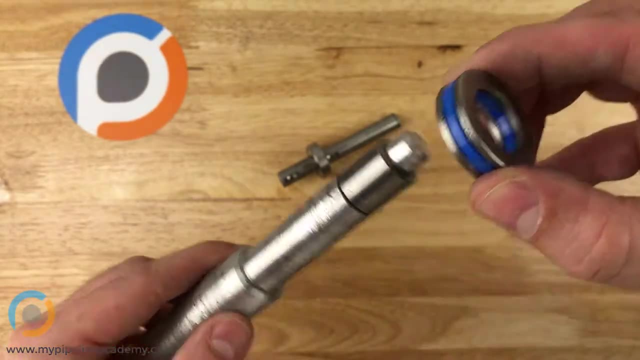 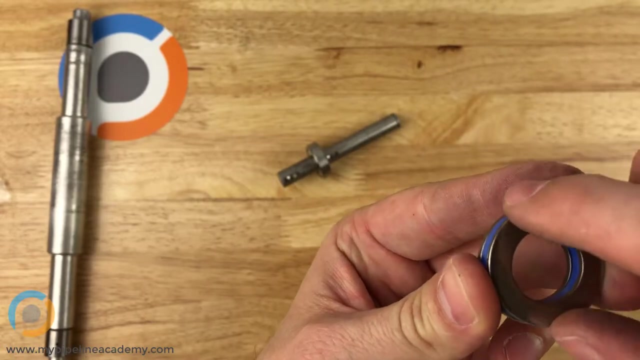 on it, putting a load on it, some force on it, but that you wanted to be able to to rotate really smoothly. I guess maybe that's the best way to explain the difference is that with a thrust washer, your, your load is is directed down into those ball bearings, like 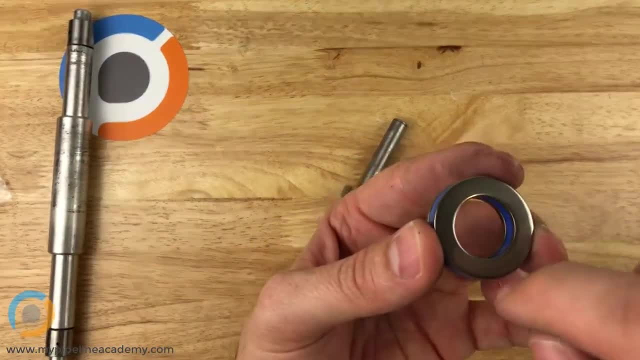 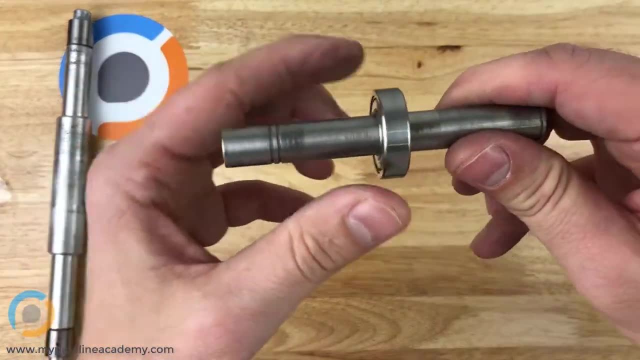 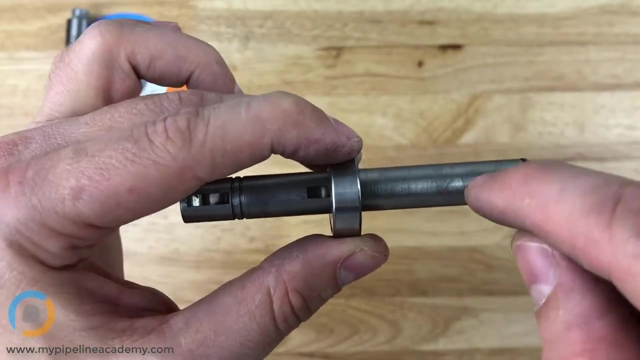 that you know, whereas down into all of the balls equally, in an equal amount, you're pushing down on it, whereas this style ball bearing you you might have your bearing, might be held in some- I don't know- part in some housing like that and you might have a load down in this direction. so it's a radial. 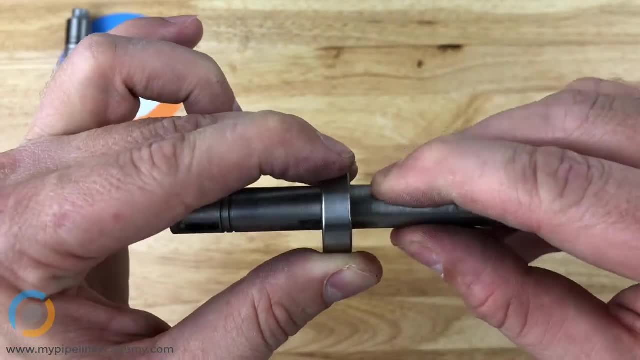 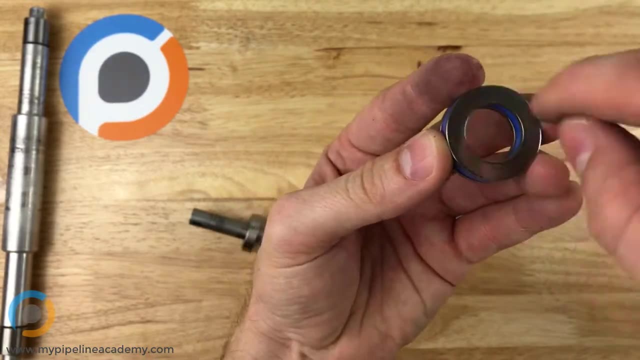 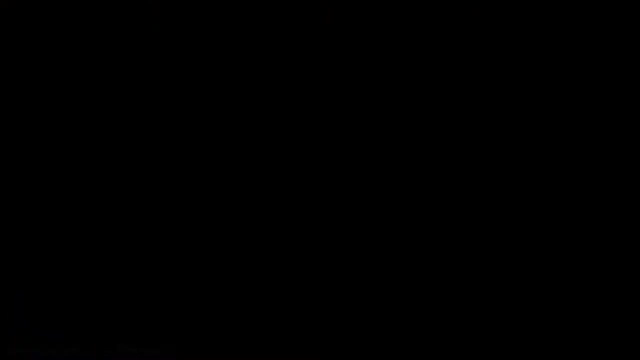 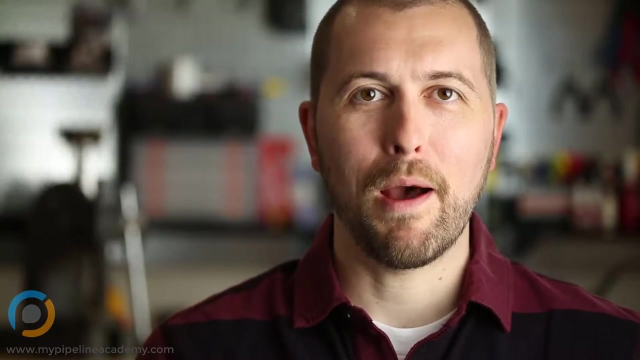 load. it's a radial load, pushing down on just a few of those balls, whereas the thrust bearing is a base load. it's pushing down on on all of those balls at the same time. so, anyway, uh, ball bearings. if you found this content helpful, consider enrolling in our signature program at mypipelineacademycom.